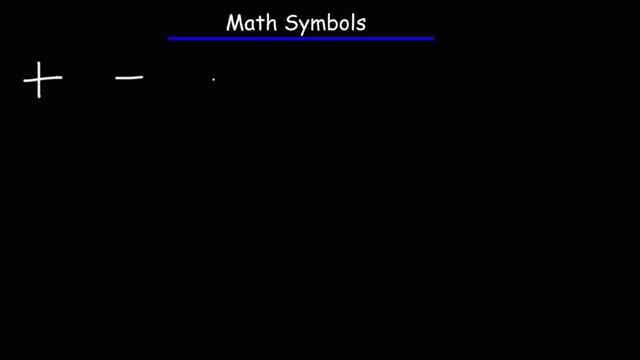 Next we have the minus sign, which is associated with subtraction, And then there's the x sign, which is multiplication, And then we have division. Now we also have the plus minus sign. So, for instance, if you see 5 plus or minus 3, it could be 5 plus 3,, which is 8,, or 5 minus 3,, which is 2.. 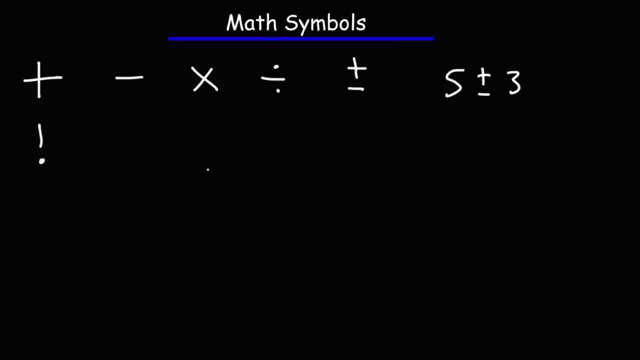 The next symbol is the factorial symbol. For instance, if we have 5 factorial, that's 5 times 4 times 3 times 2 times 1.. So we have 5 times 4 times 3 times 2 times 1.. 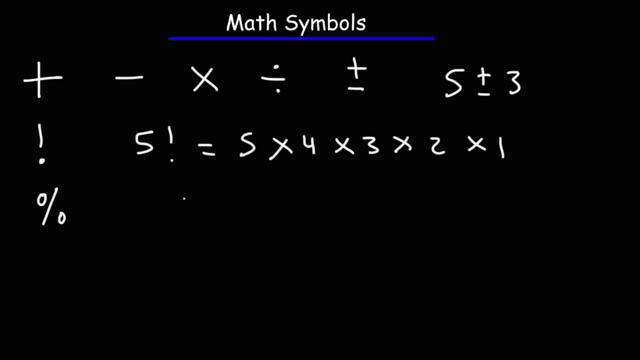 And then we have division. Next up we have percentage. Let's say, if we want to find 20% of 200.. That will be 200 times 0.20, which is 40.. Next we have the square root symbol. 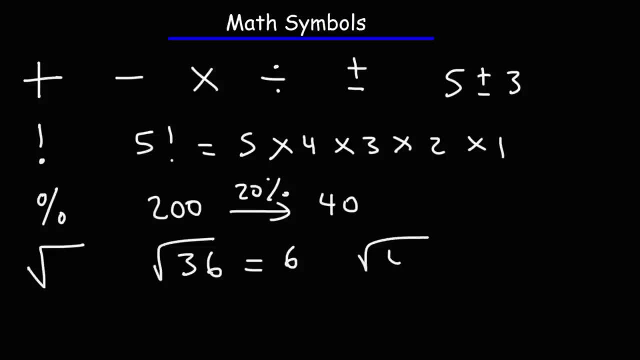 For instance, the square root of 36 is 6.. The square root of 49 is 7.. Following that, we have the cube root symbol. The cube root of 8 is 2, because 2 times 2 times 2 is 7.. 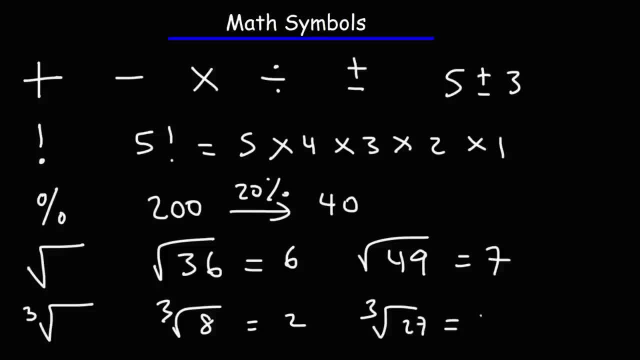 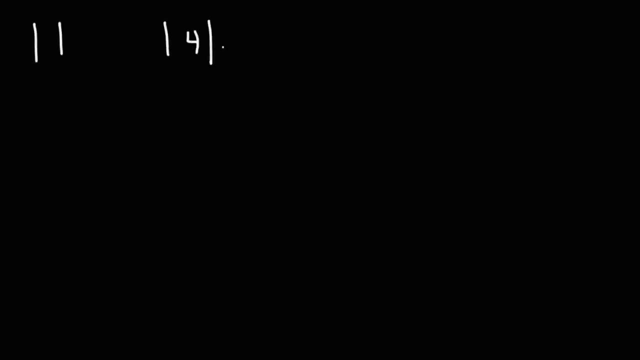 The cube root of 27 is 3, because it takes 3 3s to get to 27 when multiplied. Now the next symbol is the absolute value symbol. The absolute value of 4 is 4.. The absolute value of negative 4 is positive 4.. 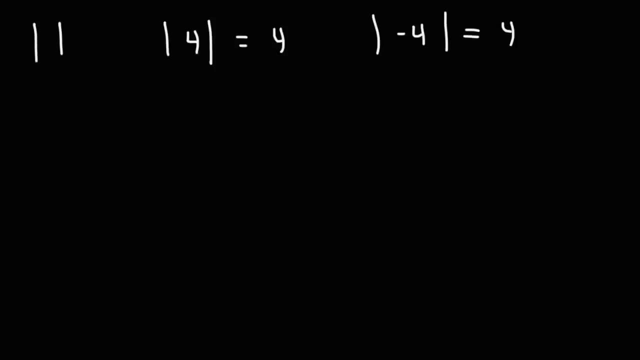 So, with the absolute value symbol, whatever is inside of it, it will always output 0 or a positive result. Now let's talk about equivalence. This sign means equal to. This sign means it is not equal to. For instance, x can be equal to 4.. 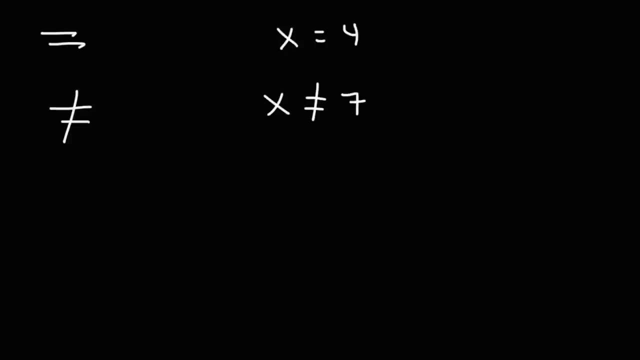 This means that x is not equal to 7.. Next, you have the approximate symbol. x may be approximately 3.46.. It could be 3.461289.. and it could keep on going. when you're rounded, it's good to use the approximation symbol now. 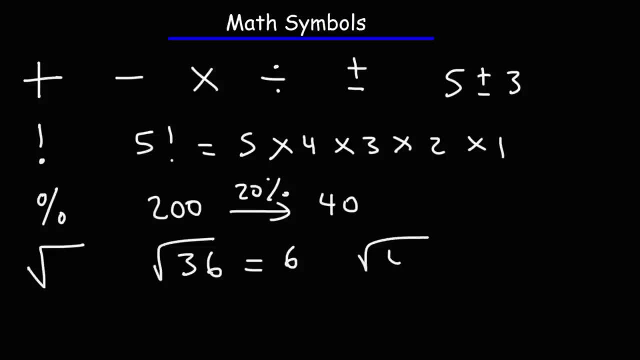 For instance, the square root of 36 is 6.. The square root of 49 is 7.. Following that, we have the cube root symbol. The cube root of 8 is 2, because 2 times 2 times 2 is 7.. 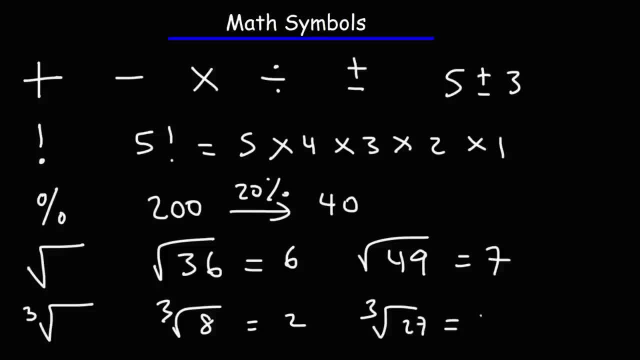 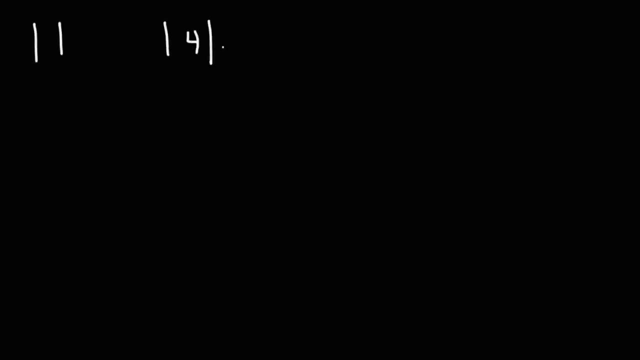 The cube root of 27 is 3, because it takes 3 3s to get to 27 when multiplied. Now the next symbol is the absolute value symbol. The absolute value of 4 is 4.. The absolute value of negative 4 is positive 4.. 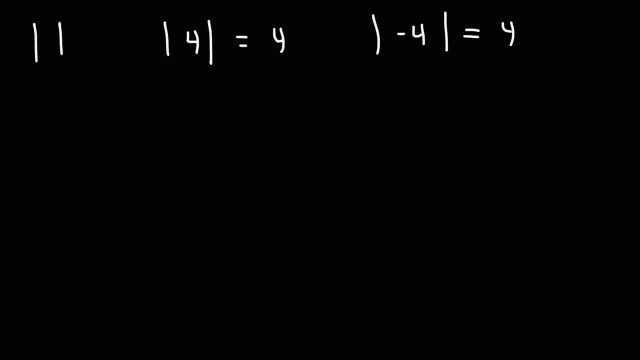 So with the absolute value symbol, whatever is inside of it, it will always output 0 or a positive result. Now let's talk about equivalence. This sign means equal 2.. This sign means it is not equal 2,, for instance. 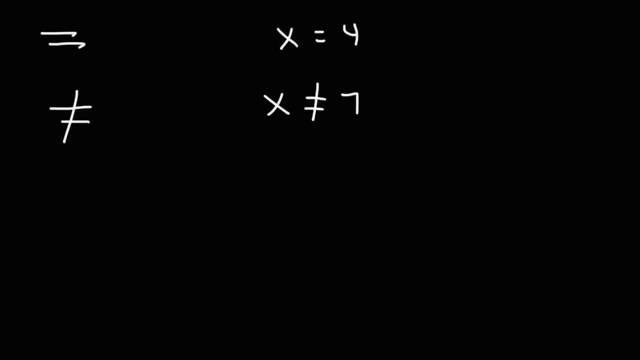 X could be equal to 4.. This means that x is not equal to 7.. Next you have the approximate symbol. X may be approximately 3.46.. It could be 3.461289.. And then you have the approximate symbol. 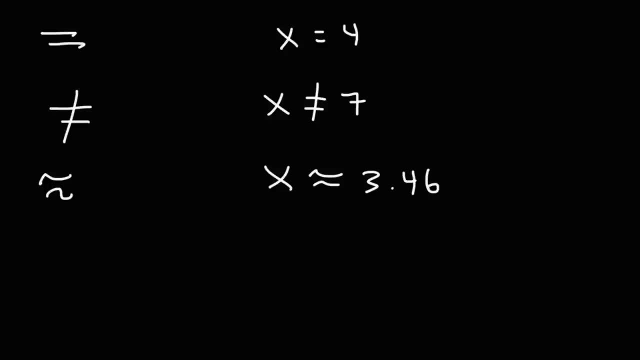 And it could keep on going. When you're rounding, it's good to use the approximation symbol. Now, this symbol means similar or is associated with similarity. For instance, you could say that triangle ABC is similar to triangle DEF. They could be similar in the sense that they have similar ratios. 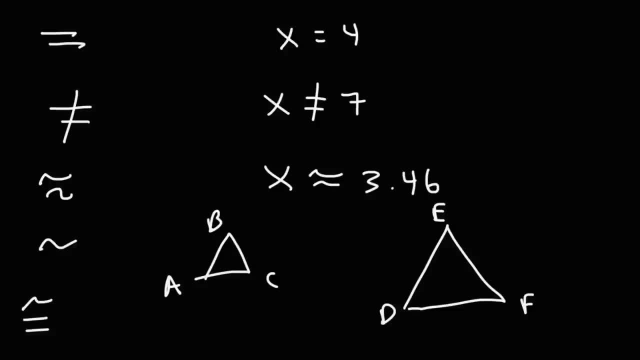 This symbol means congruent, Or triangle ABC could be congruent to triangle DEF. Now let's talk about inequalities. So this symbol means greater than and this symbol means less than. For instance, we could say that X is greater than 5, or we could say that Y is less than 3.. 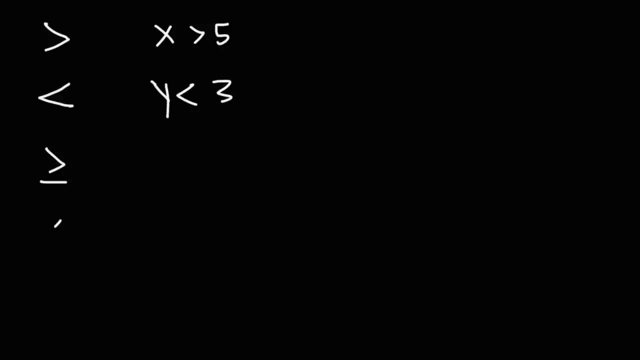 This symbol means greater than or equal to, and this one means less than or equal to. For instance, X can be equal to or greater than. This symbol means greater than 1, and Y could be less than or equal to negative 2.. 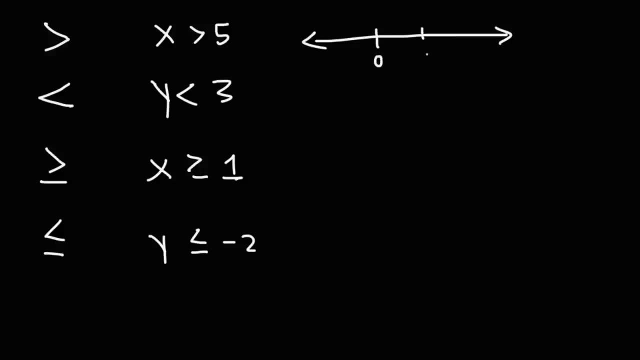 So on a number line, here's 0,, here's 5.. We would have an open circle on 5, and we would shade to the right. The open circle indicates that it doesn't equal to 5, but it's simply greater than 5.. 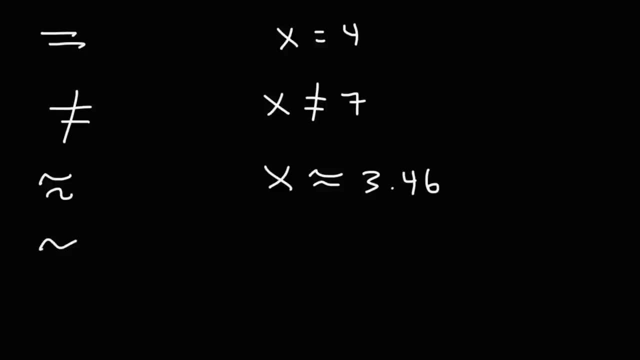 this symbol means similar or is associated with similarity. for instance, you could say that triangle ABC is similar to triangle D E F. they could be similar in a sense that they have similar ratios. this symbol means congruent. triangle ABC could be congruent to triangle D E F. now let's 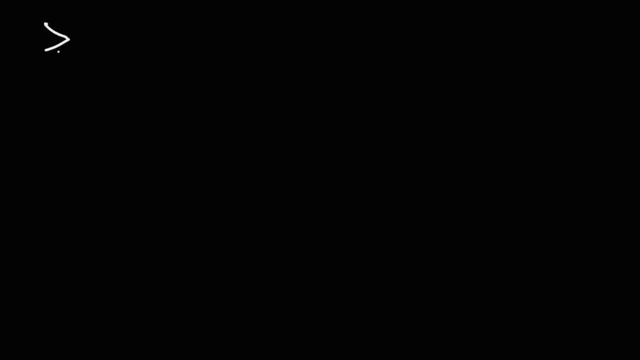 talk about inequalities. so this symbol means greater than and this symbol means less than. for instance, we could say that X is greater than 5, or we could say that Y is less than 3. this symbol means greater than or equal to, and this one means less than or equal to. for instance, X can be equal to or greater than 1. 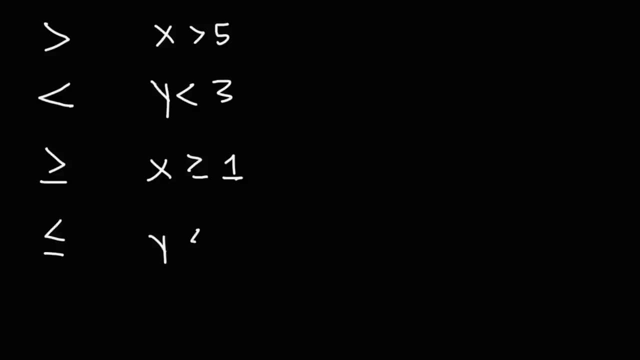 and Y could be less than or equal to negative 2. so on a number line- here's 0, here's 5- we would have an open circle on 5 and we would shade to the right. the open circle indicates that it doesn't equal to 5 but is simply greater than 5. for the next one to plot, Y is less than 3. 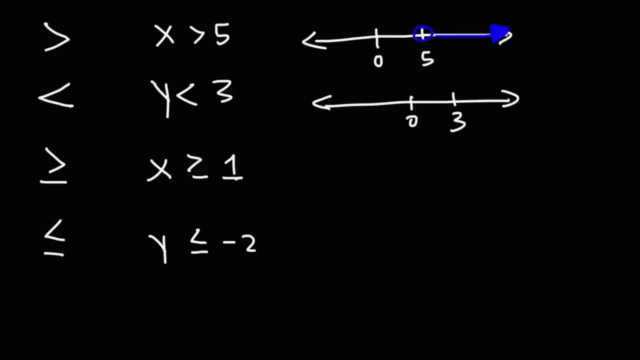 and we would show you to the left, but we still have an open circle at 3.. Next, x is equal to or greater than, 1.. Because it includes 1, we're going to have a closed circle Now for the next one, y is less than or equal to negative 2.. 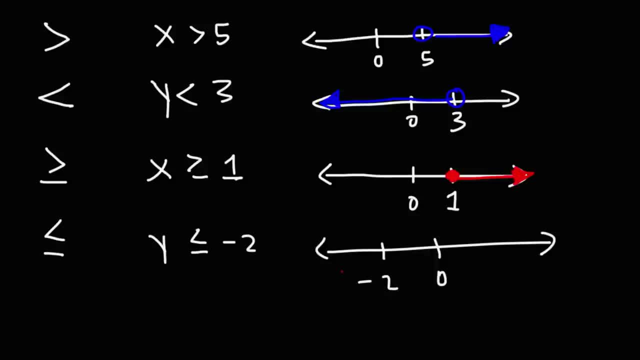 So we're going to have a closed circle at negative 2, but we're going to show you to the left, since it's less than negative 2.. So those are some inequalities that you want to be familiar with. Now there are some other ones. 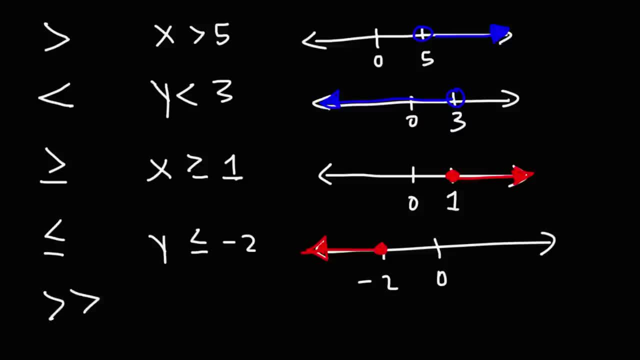 If you see two arrows pointing to the right, that means it's much greater than, For instance, let's say, x is significantly greater than 1.. That means x is a very, very large number. It's much greater than 1.. 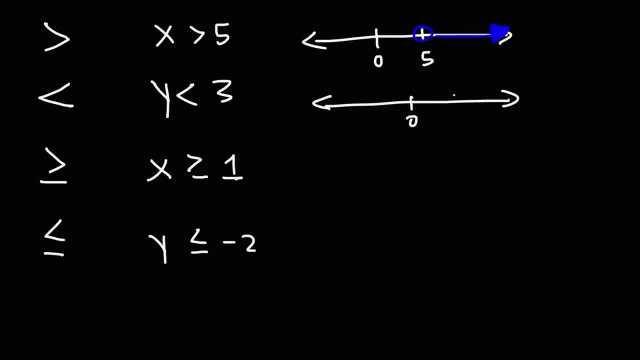 For the next one to plot: Y is less than 3, we would shade to the left, but we still have an open circle at 3.. Next, X is equal to or greater than 1.. Because it includes 1, we're going to have a closed circle. 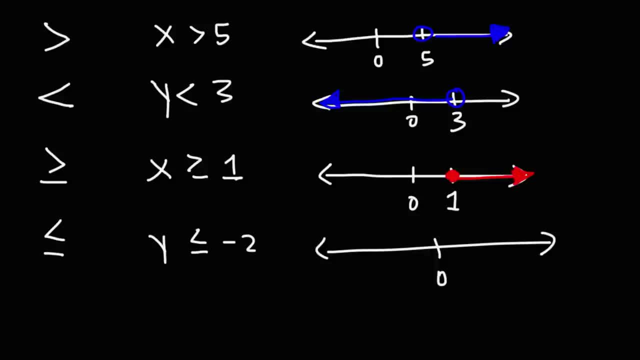 Now for the next one. Y is less than or equal to negative 2.. So we're going to have a closed circle at negative 2, but we're going to shade to the left, since it's less than negative 2.. 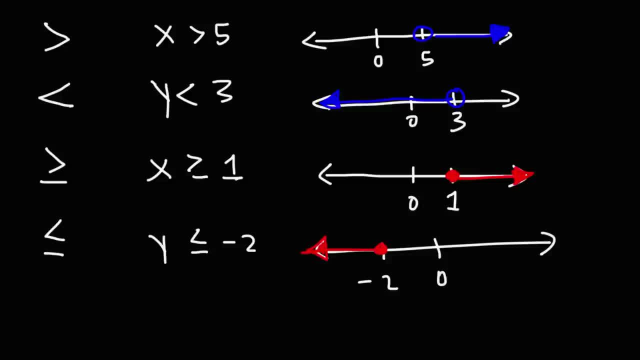 So those are some inequalities that you want to be familiar with. Now there are some other ones. If you see two arrows pointing to the right, that means it's much greater than, For instance, let's say, X is significantly greater than 1.. 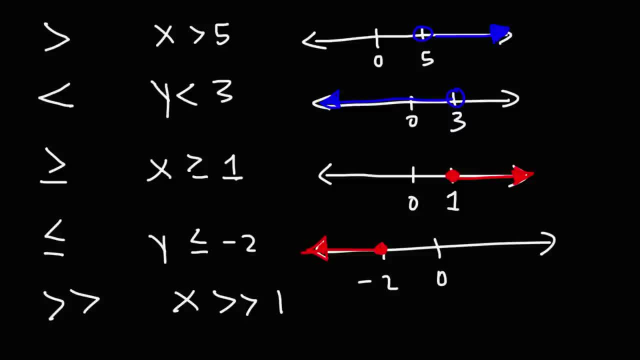 That means X is a very, very large number. It's much greater than 1.. Or you could say X is significantly greater than 1,000.. This means that Y is significantly less than some number. Maybe it's less than 0.1.. 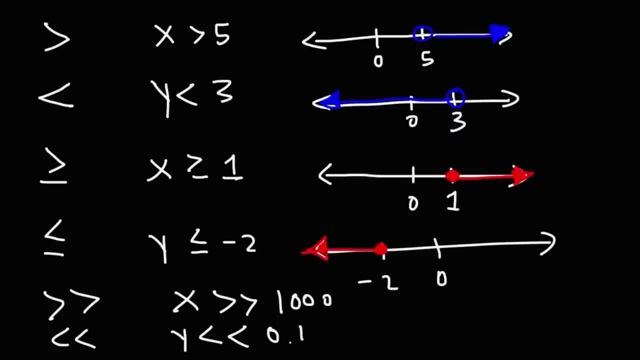 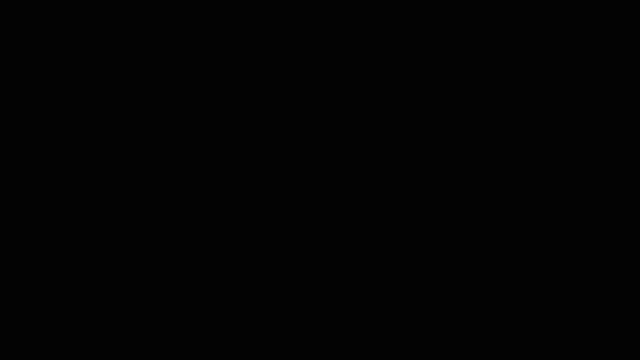 Or like, very, very like, much less than that. So when you see two arrows, it indicates extreme inequalities. Now let's talk about some math symbols that you may encounter in geometry. So if you see this symbol, it means that the two lines are perpendicular to each other. 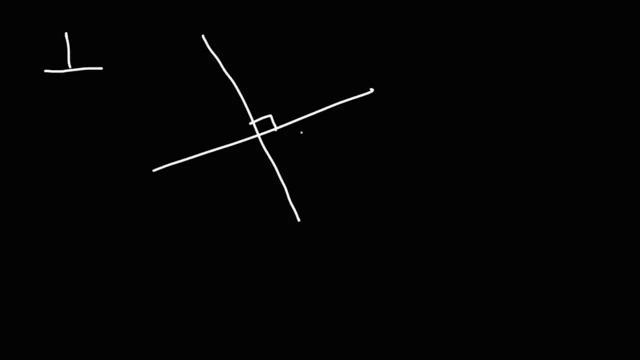 So here's a line. Here's a perpendicular line. They meet at right angles. So let's say that's line L. This is line M. You could say that line L is perpendicular to line M. This symbol means that the two lines are parallel. 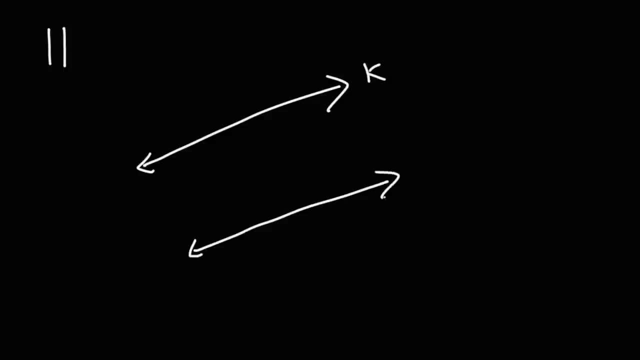 So let's say we have line K and line J. These lines are parallel. They don't intersect. So you could say that J is parallel to K. If you see this, this means line AB. If you see this with one arrow, it means ray AB. 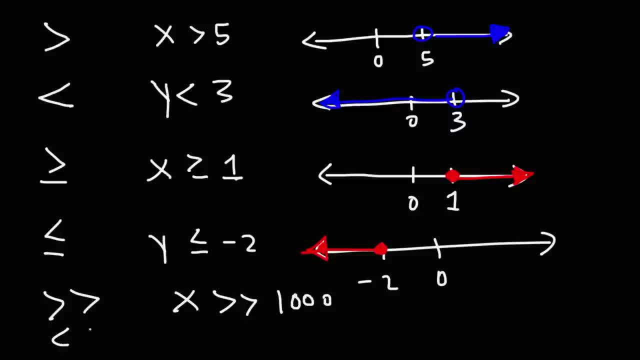 Or you could say x is less than 1.. Or x is significantly greater than 1,000. This means that y is significantly less than some number. Maybe it's less than 0.1.. Or like, very, very like, much less than that. 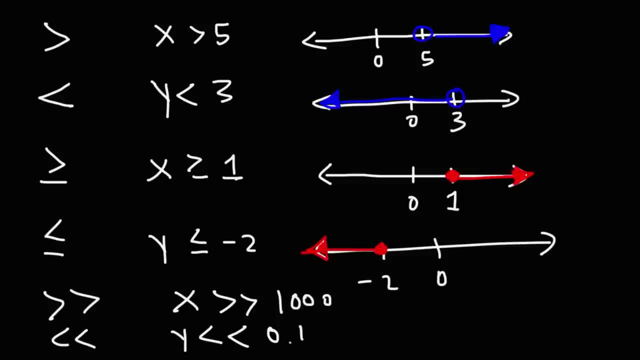 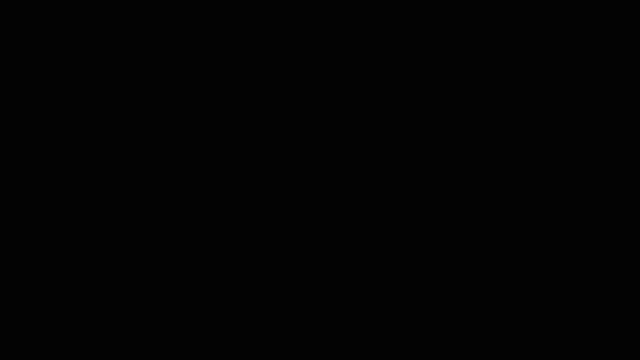 So when you see two arrows, it indicates extreme inequalities. Now let's talk about some math symbols that you may encounter in geometry. So if you see this symbol, it means that the two lines are perpendicular to each other. So here's a line, here's a perpendicular line. 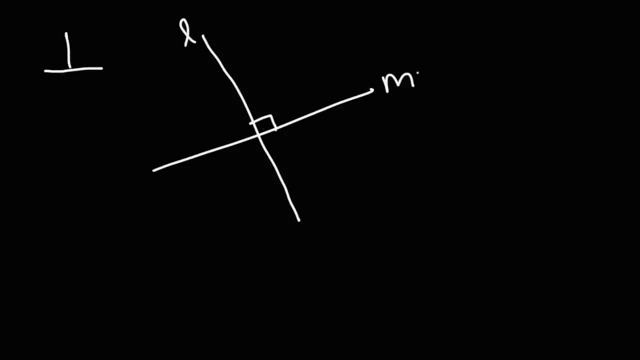 They meet at right angles. So let's say that's line L, this is line M. You could say that line L is perpendicular to line M. This symbol means that the two lines are parallel. So let's say we have line K and line J. 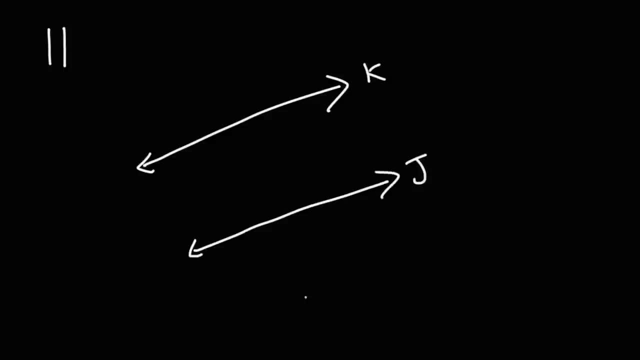 These lines are parallel, they don't intersect. So you could say that J is parallel to K. If you see this, this means line AB. If you see this with one arrow, it means ray AB. So a line can go in both directions. 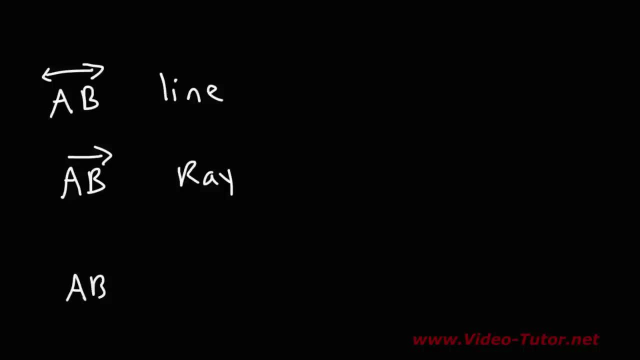 A ray points in one direction And, if you see this, this is segment AB. So this is a line, this is a ray. A ray has a beginning, but then it continues further in the other direction. A segment is limited in length. 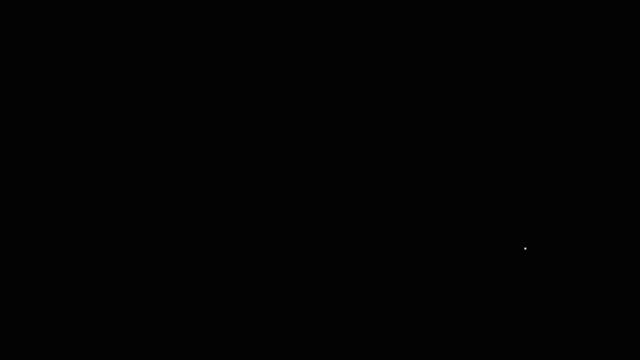 It has a beginning and an end. If you see this symbol, it means a right angle. Think of a right triangle. You'll see this 90 degree right angle there. This means the angle is a Q. This means the angle is a Q. 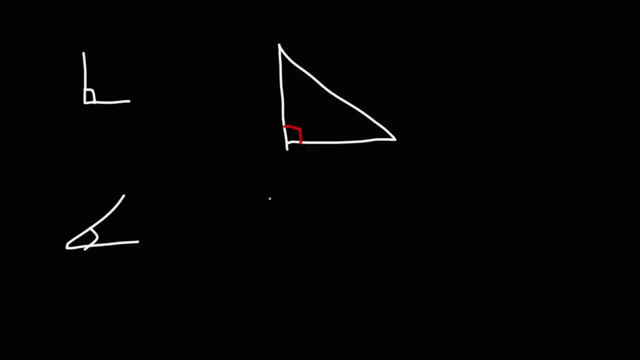 Or it's less than 90 degrees, And this symbol means degrees. So if you see 80 with this, that means 80 degrees or 70 degrees. Sometimes you may see that with reference to temperature, It's 75 degrees Fahrenheit or 64 degrees Celsius. 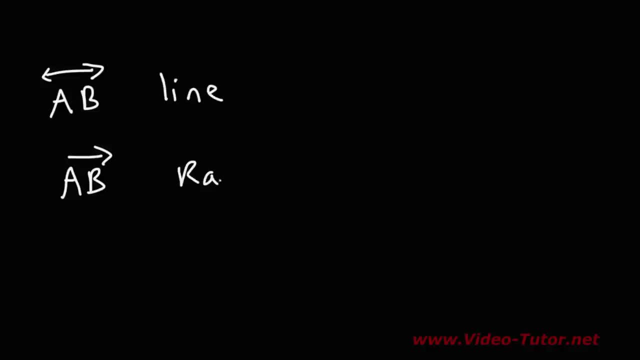 So a line can go in both directions. A ray points in one direction And, if you see this, this is segment AB. So this is a line, This is a ray. A ray has a beginning, but then it continues forever in the other direction. 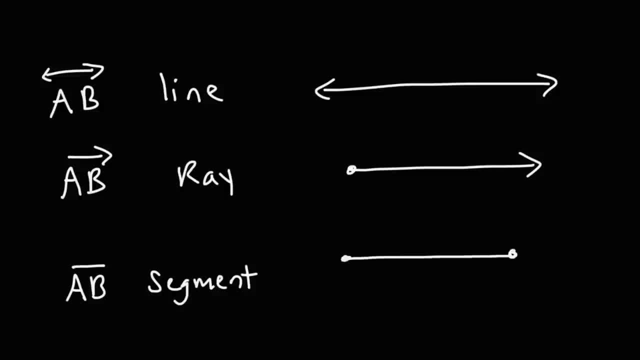 A segment is limited in length. It has a beginning and an end. If you see this symbol, it means a right angle. Think of a right triangle. You'll see this 90 degree right angle there. This means the angle is a Q or it's less than 90 degrees. 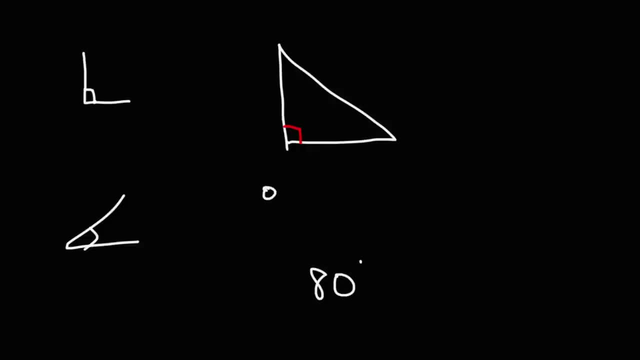 And this symbol means degrees. So if we see 80 with this, That means 80 degrees or 70 degrees. Sometimes you may see that with reference to temperature, It's 75 degrees Fahrenheit or 64 degrees Celsius. Now, if we see this symbol, it means proportional to 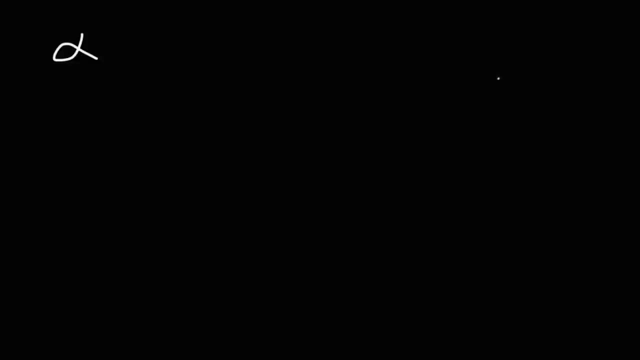 So, for instance, let's say: if we have an equation, Let's say it's a gravitational force, Let's say it's GM1. M2 over R squared, So we can say that the gravitational force is proportional to the mass of the planet. 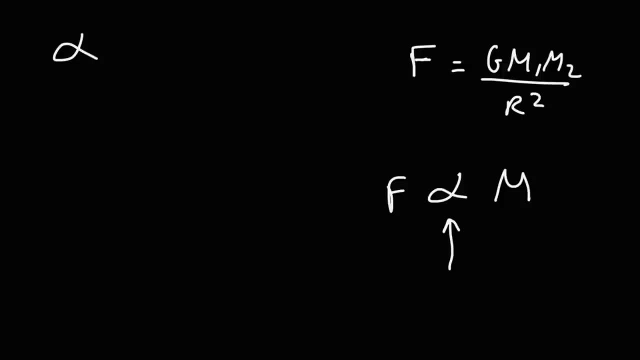 So this simply relates two variables together. Now, when you see a colon in math, it represents a ratio. For instance, this means 5 to 3.. Maybe there's 5. For every 3 girls in the class. 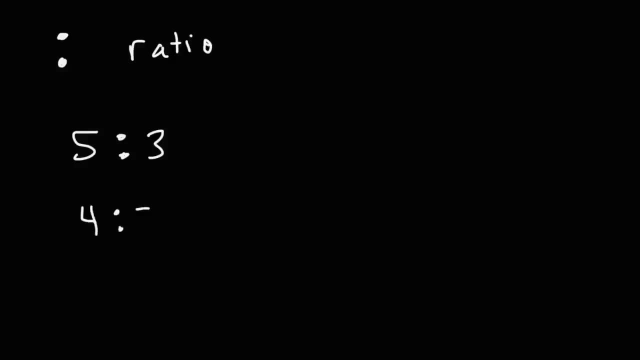 Or maybe there's 4 blue marbles for every 7 red marbles in the back. So when you see a colon, it indicates a ratio. If you see the letter I in math, this means imaginary. It's an imaginary number. 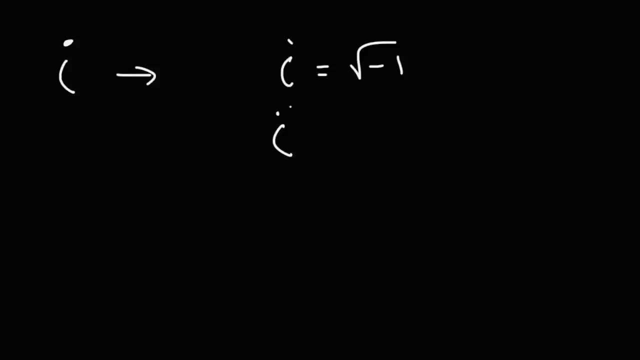 I is equal to the square root of negative 1. I squared is negative 1. I to the third is negative. I. I to the fourth is equal to positive: 1.. Now the next symbol which looks like a U. this symbol means union. 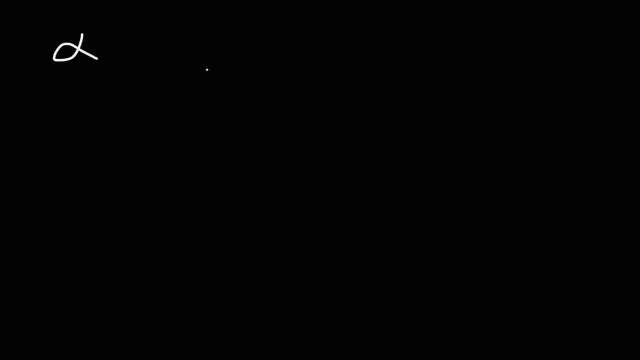 Now, if you see this symbol, it means proportional to. So, for instance, let's say: if we have an equation. For instance, let's say: if we have an equation- Gravitational force, let's say it's GM1M2 over R squared. 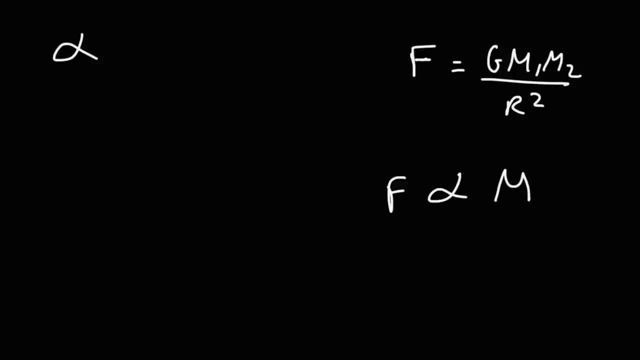 So we can say that the gravitational force is proportional to the mass of the planet. So this simply relates two variables together. Now, when you see a colon in math, it represents a ratio. Now, when you see a colon in math, it represents a ratio. 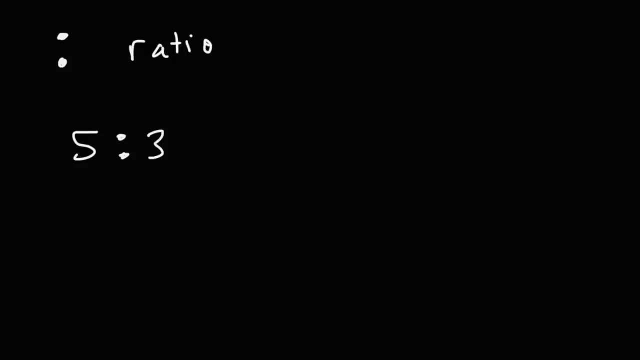 For instance, this means 5 to 3.. Maybe there's five boys for every three girls in the class. Maybe there's four blue marbles for every seven red marbles in the bag. Maybe there's four blue marbles for every seven red marbles in the bag. 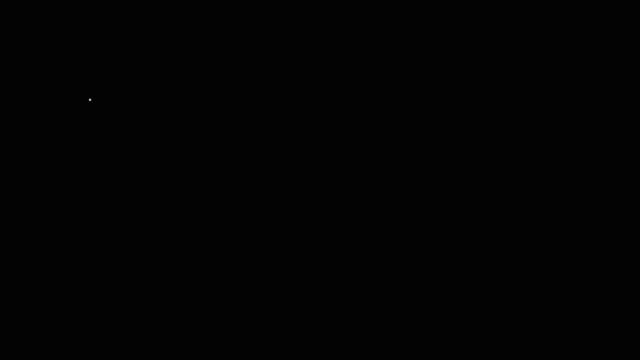 So when you see a colon it indicates a ratio. If you see the letter i in math this means imaginary. It's an imaginary number is equal to the square root of negative one. I squared is negative one. I to the third is: 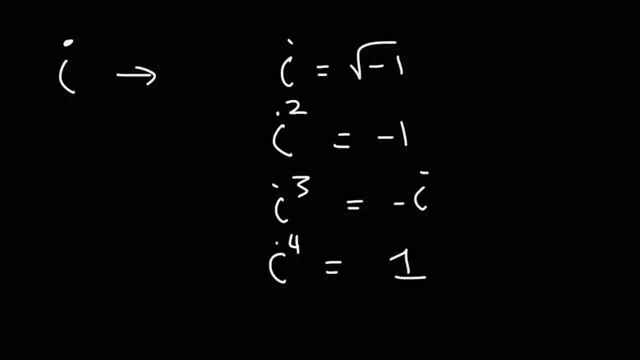 negative I. I to the fourth is equal to positive one. Now the next symbol, which looks like a U. this symbol means union. Typically, you're joining two things together. So let's say, if you have a number line and you need to find the domain of a function, which is a very common situation in math- 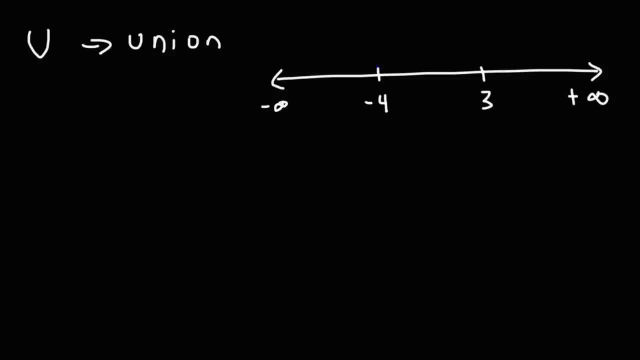 and let's say the domain represents everything that's shaded in blue. So the domain would be negative infinity to negative four. Since we have an open circle at negative four, we're going to use a parenthesis. Now we want to combine it with this section, So we: 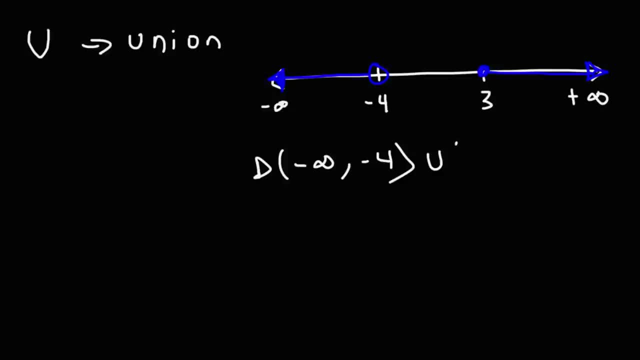 want to combine those two, So we would use the union symbol to connect them together. Now three is included, so we're going to use a parenthesis, So we're going to use a bracket to include three, and then it's going to go to a positive. 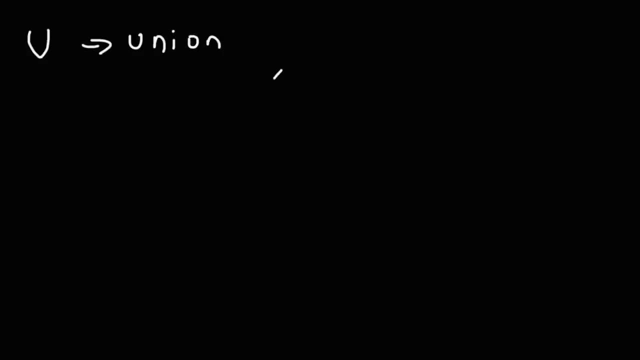 Typically you're joining two things together. So let's say, if you have a number line And you need to find the domain of a function- which is a very common situation in math- And let's say the domain represents Everything that's shaded in blue. 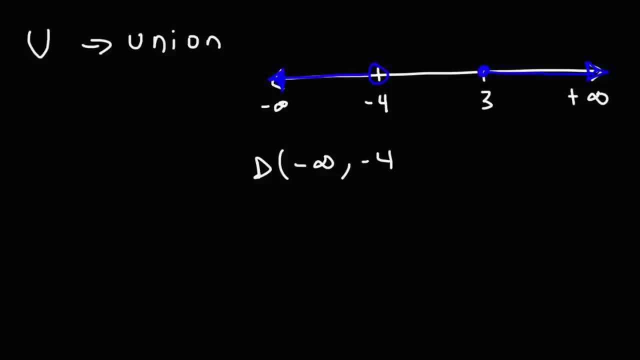 So the domain would be negative infinity to negative 4.. Since we have an open circle at negative 4, we're going to use a parenthesis. Now we want to combine it with this section. So we want to combine those two. 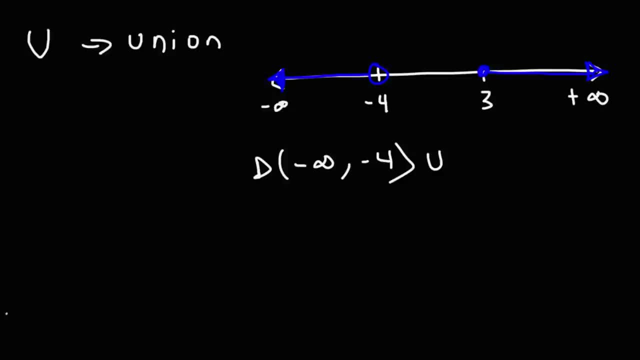 So we would use the union symbol to connect them together. Now 3 is included, so we're going to use a bracket to include 3. And then it's going to go to a positive infinity. So U represents union. 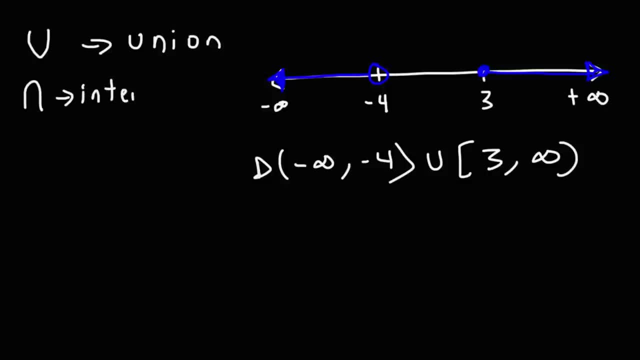 This means intersection. Intersection is where the two groups, where they intersect or they have some kind of commonality. So let's say, if you have two Venn diagrams, This is A, B and A and B share some common value. 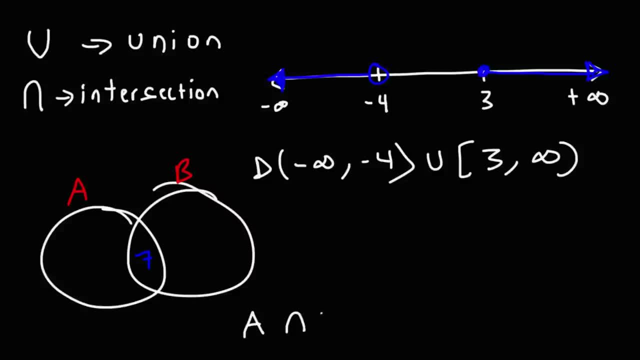 So 7 would be part of the intersection of A and B, Because it's found in both. That's where they intersect. Now, the next symbol that we need to talk about is this: The interval a to b using parentheses. this is an open interval. Now using brackets: 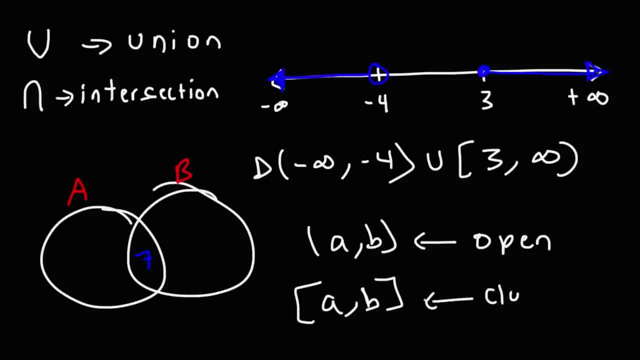 this interval from a to b. that's a closed interval. So notice what we did with negative four: Because we have parentheses, we use an open circle, Whereas for three we had a bracket. so we use a closed circle Because three is on the interval. negative four is: 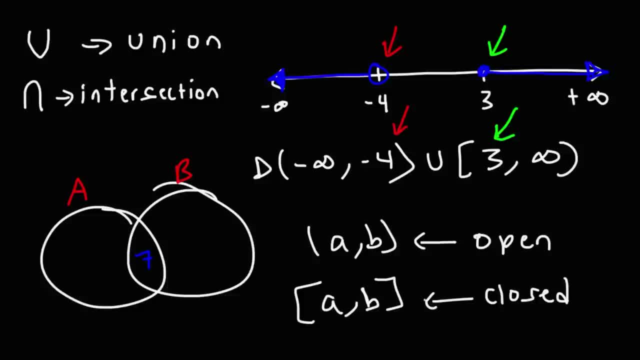 not. So that's the difference between an open interval and a closed interval. Now, there's another symbol here that I haven't officially mentioned, but I kind of mentioned already, And that is the affinity symbol. So whenever you see this, that is infinity. 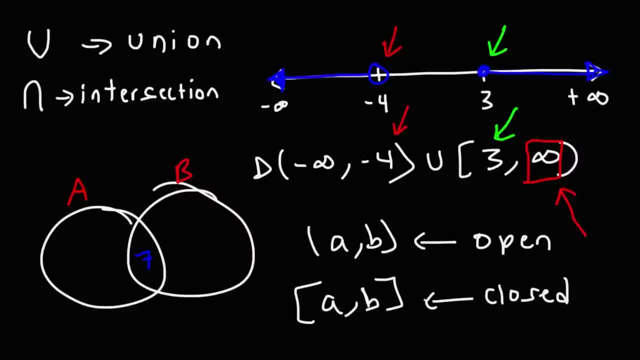 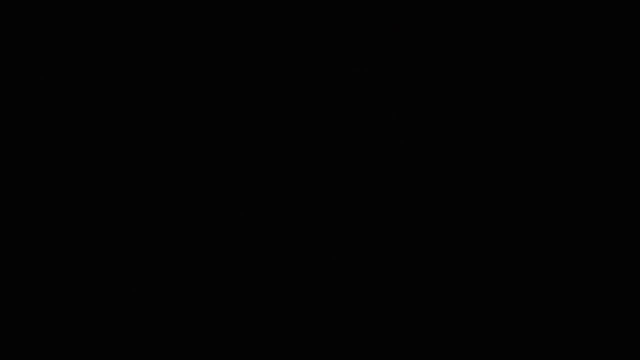 That means it's a very, very high number. A very, very high, non-specific number is a better way to describe it. Now, if you're taking calculus, a symbol that you're going to see is the integral symbol. It's associated with accumulation, but that's a topic for another day. Now let's move on. 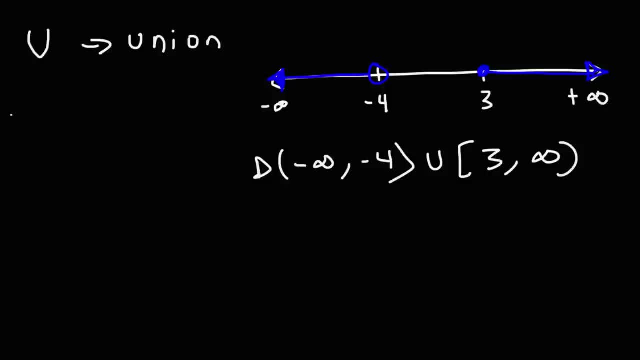 infinity. So U represents union. This means intersection. Intersection is where the two groups, where they intersect or they have some kind of commonality. So let's say, if you have two Venn diagrams, this is A, B, and A and B share some common value. So seven would be part. 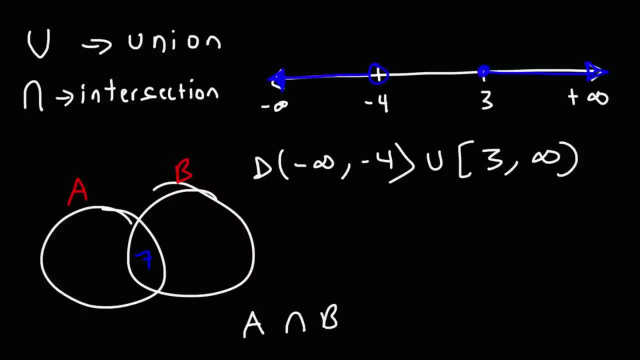 of the intersection of A and B, Because it's found in both. That's where they intersect. Now, the next symbol that we need to talk about is this: The interval A to B. using parentheses, this is an open interval. Now, using brackets, this interval from A to B: that's a closed interval. 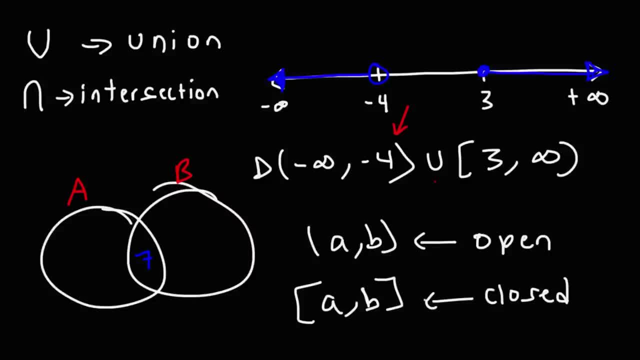 So notice what we did. So we did it with negative four. Because we have parenthesis, we use an open circle, Whereas for three we had a bracket. so we use a closed circle Because three is on the interval. negative four is not. 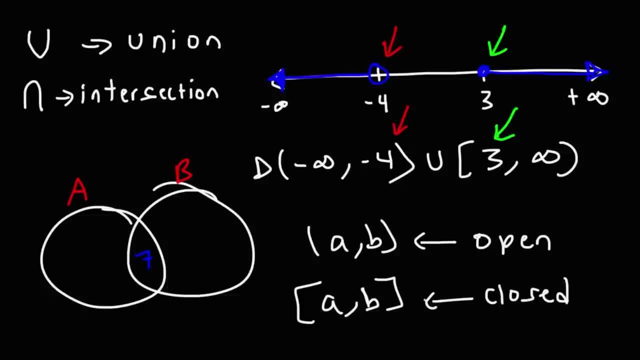 So that's the difference between an open interval and a closed interval. Now, there's another symbol here that I haven't officially mentioned, but I kind of mentioned already, And that is the affinity symbol. So whenever you see this, that is infinity. 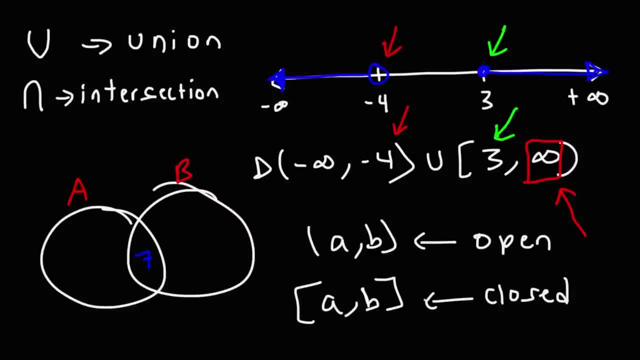 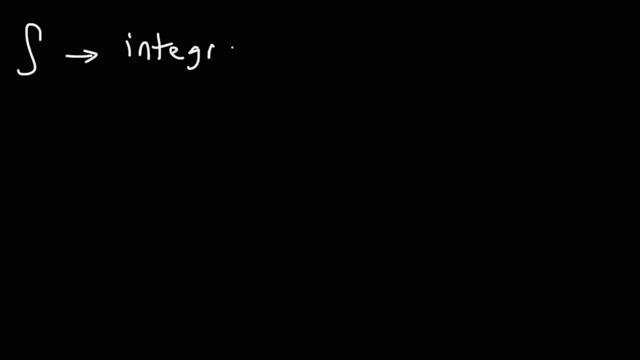 That means It's a very, very high number. a very, very high, nonspecific number is a better way to describe it. Now, if you're taking calculus, a symbol that you're going to see is the integral symbol. It's associated with accumulation, but that's a topic for another day. 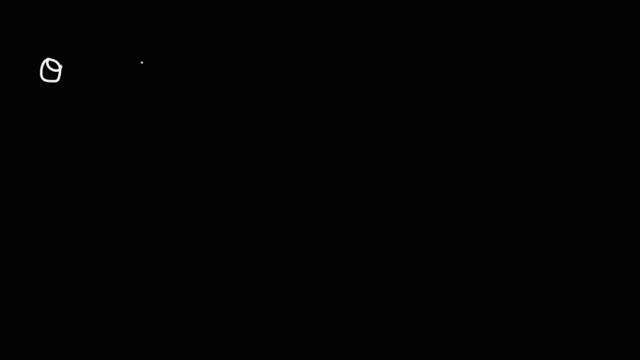 Now let's move on to angles. So this is a very common angle. you'll see, This angle is theta. So think of like sine theta or cosine theta, Or if you have a triangle, the angle in the triangle will be theta. 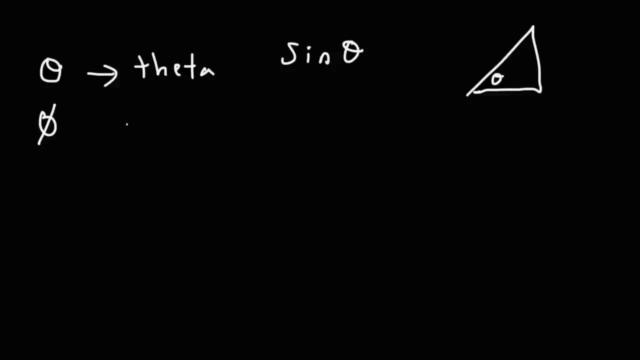 Now there's another angle which is typically complementary to theta, and this is phi. So perhaps you're dealing with vectors, and let's say you have the x-axis, the y-axis and you have a vector Pointing in this direction. 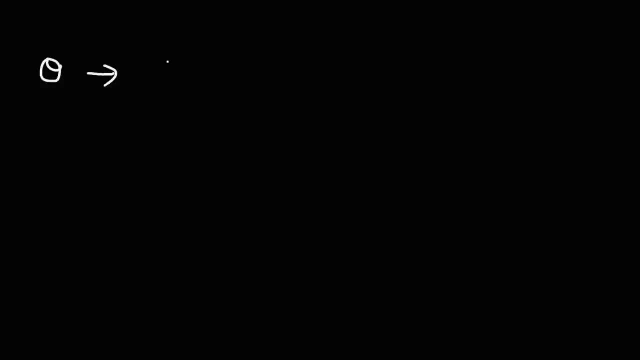 to angles. So this is a very common angle. you'll see, This angle is theta. So think of like sine theta or cosine theta, Or if you have a triangle, the angle in the triangle will be theta. Now there's another angle which is typically complementary to theta. 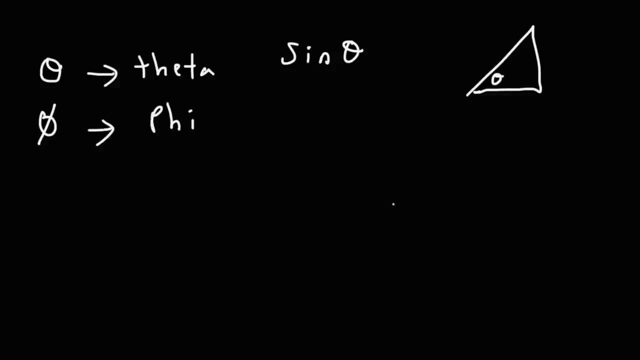 and this is phi. So perhaps you're dealing with vectors. and let's say you have the x-axis, the y-axis and you have a vector pointing in this direction. Now, this angle relative to the x-axis or between the x-axis and the y-axis is a vector. So if you have a vector, 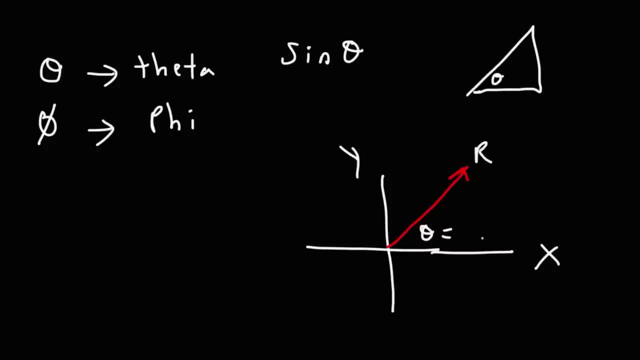 in the x-axis and the vector. we'll call this vector r. that angle may be 50 degrees. The other angle between the vector and the y-axis- this is typically phi, but it can vary. but sometimes you'll see the other angle is phi and that's usually complementary to. 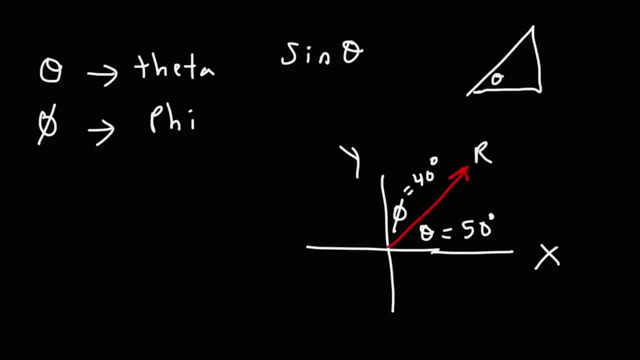 theta, So this one is going to be 40 degrees Now. sometimes you may see angles represented as alpha. That's part of the Greek alphabet. Some angles will be represented as beta In trig. sometimes you'll see some indifference formulas like sine alpha, cosine, beta, And then you have gamma, another Greek alphabet. 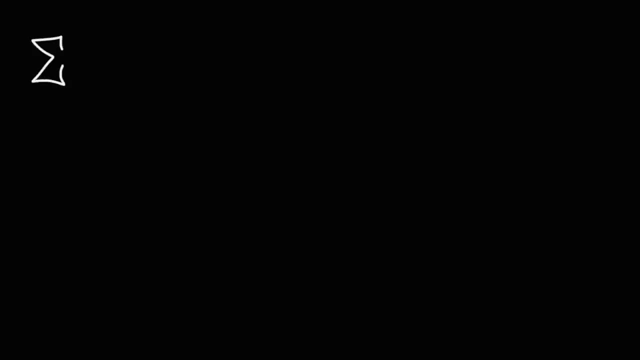 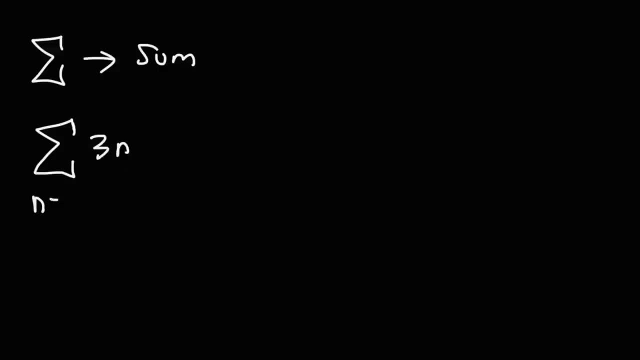 I have 3n from n equal 1 to 5.. What this means is: if I plug in 1, I get 3.. If I plug in 2,, I get 6.. If I plug in 3,, I get 9.. 4, I get 12.. 5, I get 15.. So you start here, you stop. 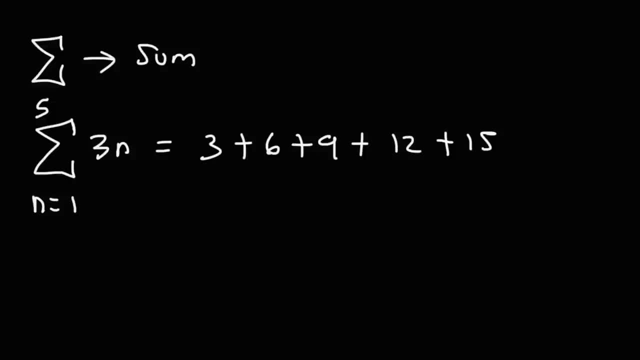 at the fifth term, and the sigma sign means summation, meaning you add up all the terms. So this answer will be the sum of those five numbers. So that's 9 plus 9, which is 18 plus 12.. 18 plus 12 is 30, plus 15 is 45. So the value of this expression is 45. So 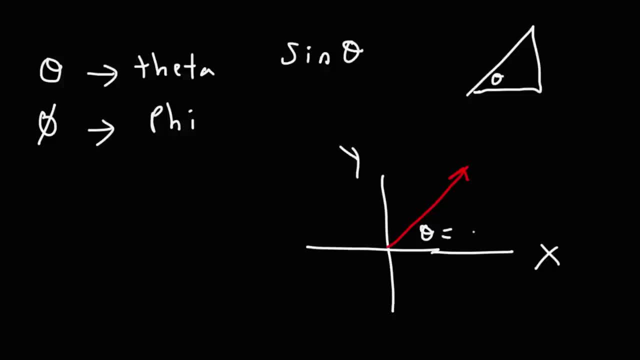 Now this angle relative to the x-axis, or between the x-axis and the vector, we'll call this vector r. that angle may be 50 degrees. The other angle between the vector and the y-axis, this is typically phi, but it can vary, but sometimes you'll see the other angle is phi. 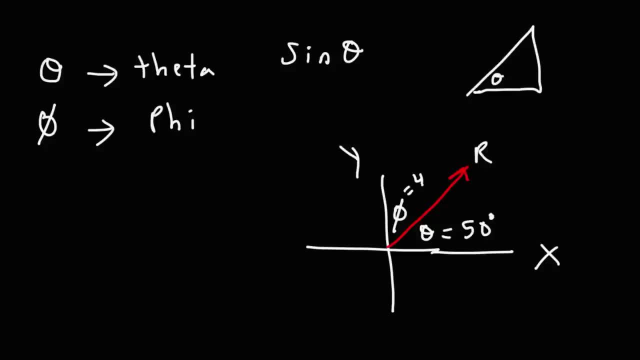 And that's usually complementary to theta. So this one is going to be 40 degrees Now. sometimes You may see angles represented as alpha. That's a part of the Greek alphabet. Some angles will be represented as beta In trig. sometimes you'll see some indifference formulas like sine alpha, cosine, beta. 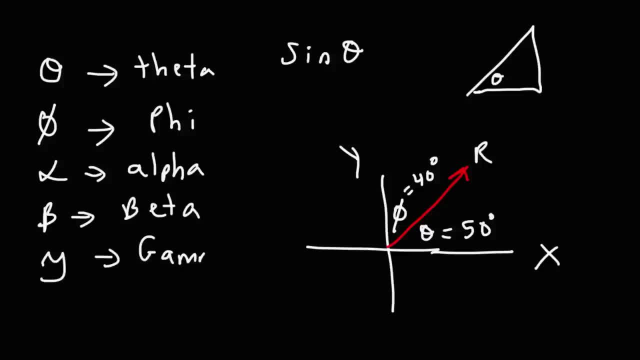 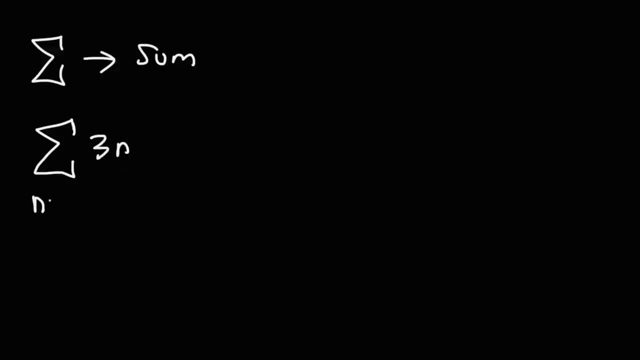 And then you have gamma, Another Greek alphabet, And then there's the Greek alphabet sigma. Sigma corresponds to sum. So for instance, let's say I have the summation of 3n from n equal 1 to 5.. What this means is if I plug in 1, I get 3.. 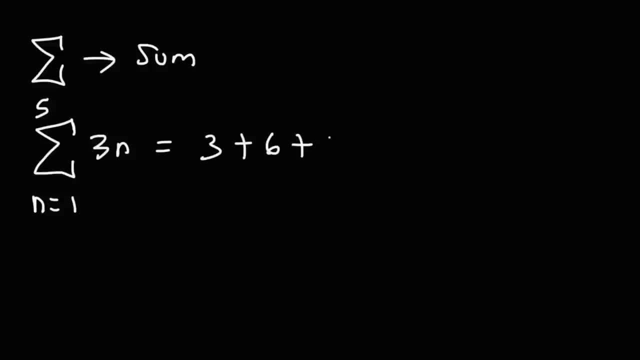 If I plug in 2,, I get 6.. If I plug in 3,, I get 9.. 4, I get 12.. 5, I get 15.. So you start here. You stop at the fifth turn. 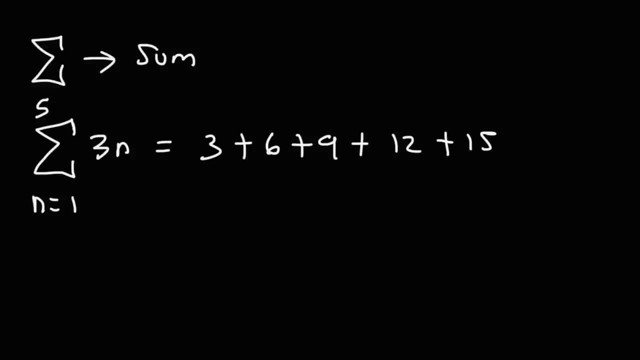 And the sigma sign means summation, Meaning you add up all the terms. So this answer will be the sum of those five numbers, So that's 9 plus 9, which is 18, plus 12.. 18 plus 12 is 30, plus 15 is 45.. 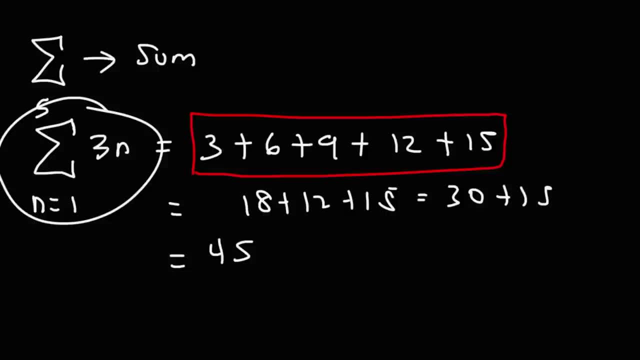 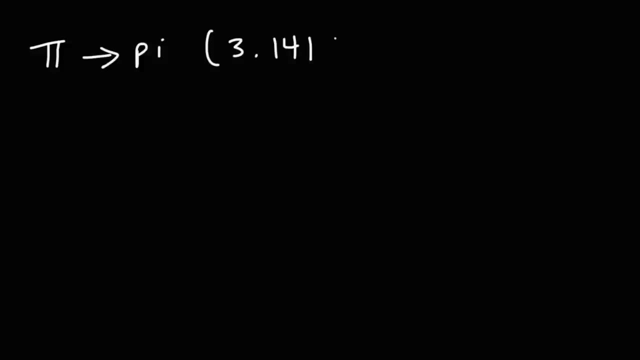 So the value of this expression is 45. So anytime you see sigma, it means sum or summation. Next up we have the symbol pi. Pi is 3.14159, with some other numbers after that, But perhaps you've seen pi in this formula. 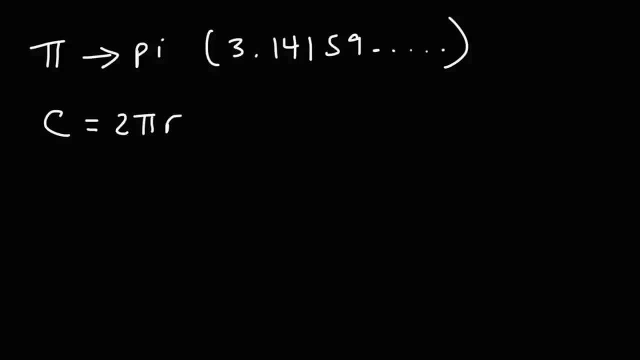 Circumference is 2 pi r. That's the circumference of a circle, or the area of a circle, pi r squared. Typically, when you're dealing with circles, you have pi in it. The next symbol is delta. Now you might see delta in two forms. 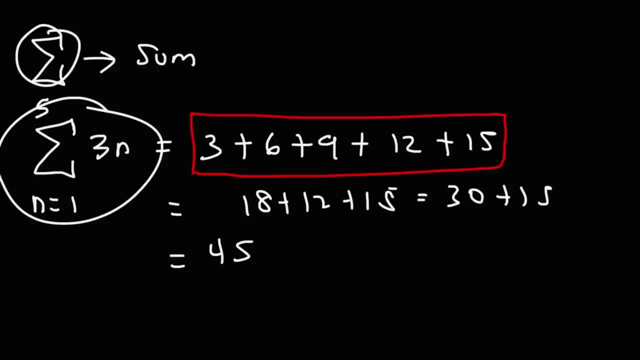 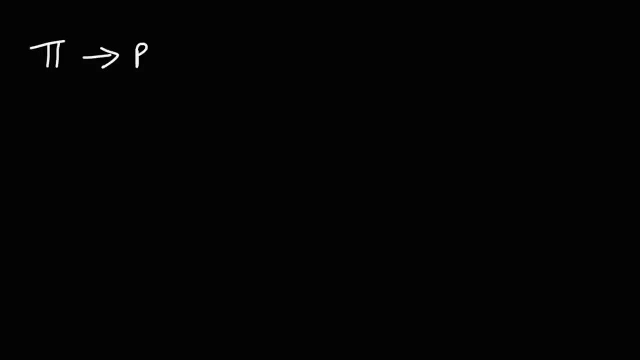 anytime you see sigma, it means sum or summation. Next up we have the symbol pi. Pi is 3.14159, with some other numbers after that, But perhaps you've seen this before, So if you've seen this before, you've seen this before. So if you've. 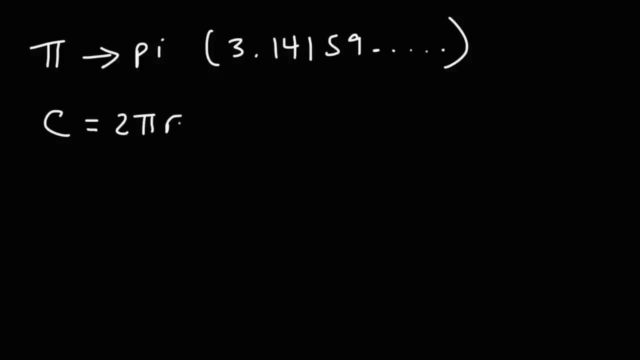 seen this before. you've seen this before, So if you've seen this before, you've seen this before. So you've seen pi. in this formula, Circumference is 2 pi r, That's the circumference of a circle. 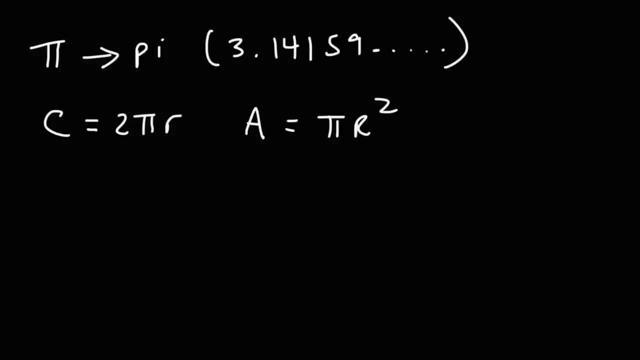 or the area of a circle, pi r squared. Typically, when you're dealing with circles, you have pi in it. The next symbol is delta. Now you might see delta in two forms. You might see it as a triangle. In this case, this represents change. So delta x, that's the change in x. 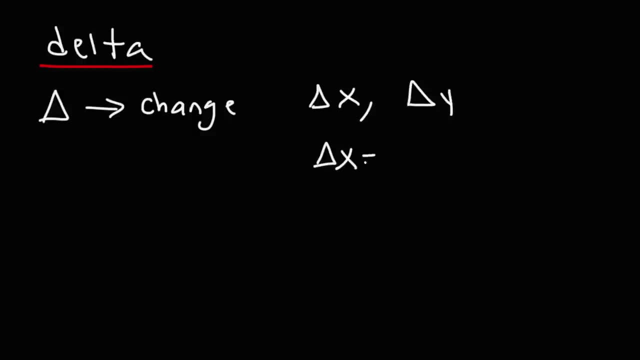 or delta y. the change in y Delta x might be the difference between two x values: x2 minus x1.. Delta y could be the final y value minus the initial y value, but it represents the change in something. Now you might see delta also in the form of a Greek symbol, So this also means delta. 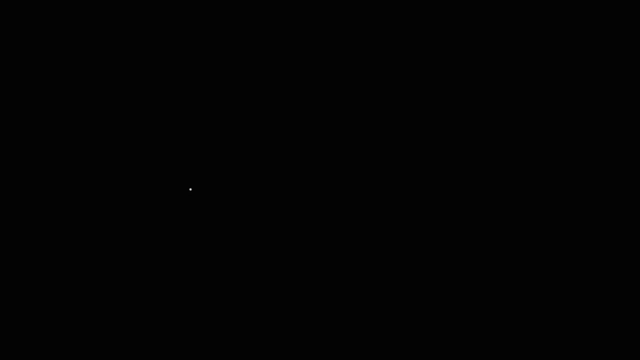 this symbol is the greek alphabet lambda, and you might encounter this when in chemistry or physics, when you're talking about electromagnetic radiation, especially light. for instance, the speed of light is equal to the wavelength times the frequency. c is the speed of light, which is three times ten to the eight meters per second. lambda represents the wavelength measured in. 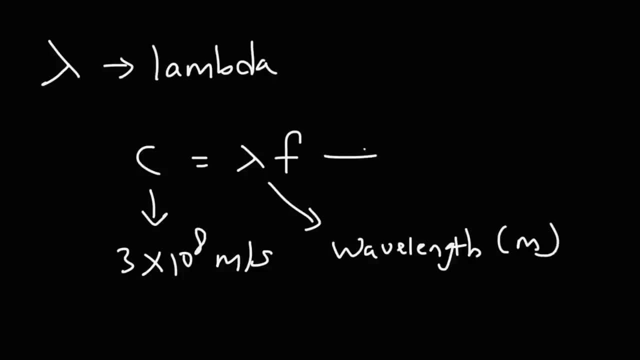 meters, and f is the frequency measured in hertz or one over seconds. so that's where lambda comes into play. typically, you'll see it represented as the wavelength of light or some form of electromagnetic radiation. the next greek symbol is rho. if you're taking physics, you might see this in when you're dealing with gauge pressure, where 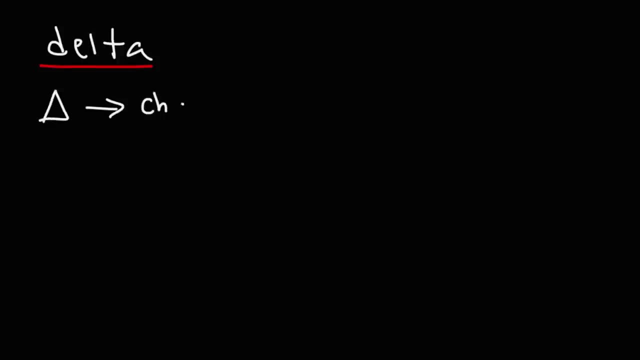 You might see it as a triangle. In this case this represents change. So delta x, that's the change in x, or delta y, the change in y. Delta x might be the difference between two x values: x2 minus x1.. 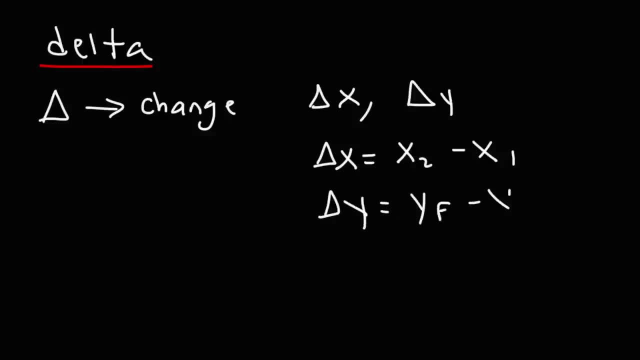 Delta y could be the final y value minus the initial y value, But it represents the change in something. Now you might see delta also in the form of a Greek symbol, So this also means delta. This symbol is the Greek alphabet lambda. 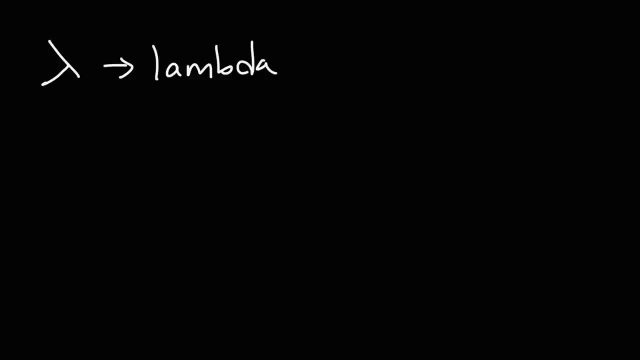 And you might encounter this in chemistry or physics when you're talking about electromagnetic radiation, especially light. For instance, the speed of light is equal to the wavelength times the frequency. C is the speed of light, which is 3 times 10 to the 8 meters per second. 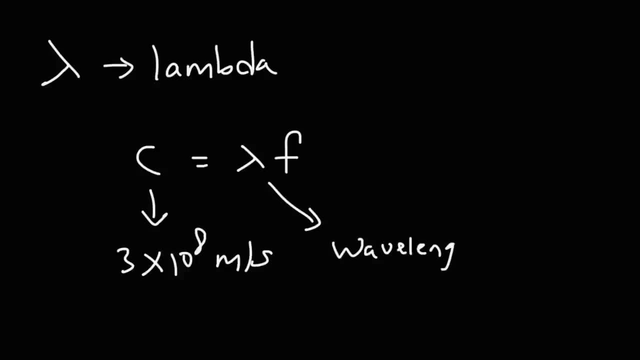 Lambda represents the wavelength. Lambda represents the wavelength measured in meters And f is the frequency measured in hertz or 1 over seconds. So that's where lambda comes into play. Typically you'll see it represented as the wavelength of light or some form of electromagnetic radiation. 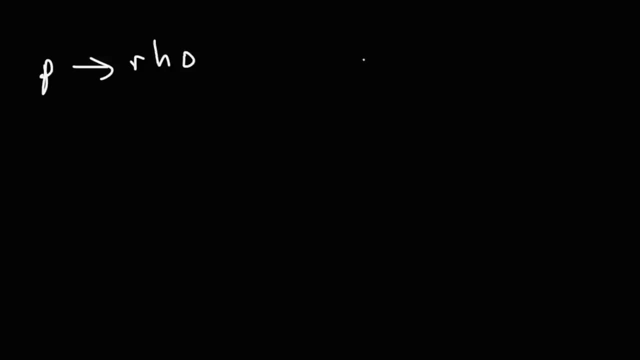 The next Greek symbol is rho. If you're taking physics, you might see this when you're dealing with gauge pressure, Where it's equal to rho- gravitational acceleration times height. So in this case, rho represents density. So in this particular formula, it's the density of a fluid. 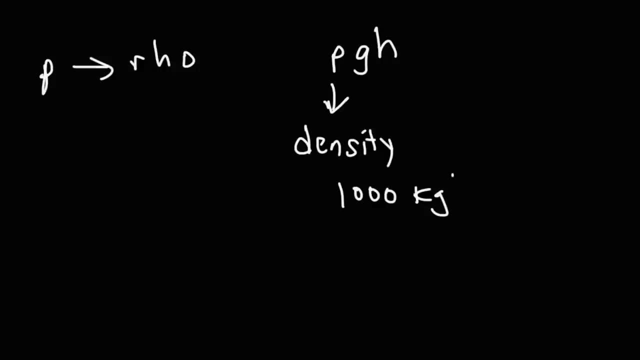 The density of water is 1000 kilograms per cubic meter. That's in physics, but in chemistry it's 1 gram per milliliter. The last symbol we're going to talk about is the omega symbol. In physics you might see this as angular frequency. 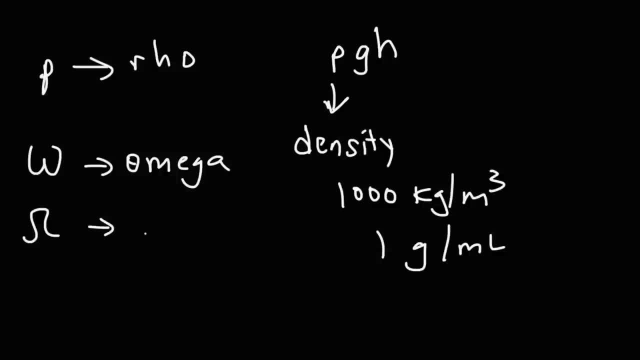 And you may also see the omega symbol in this form. When it comes to electricity, this is the unit of resistance, which is ohms. So those are some common symbols that you'll encounter when dealing with math And also when you're dealing with the math part of sciences like chemistry and physics.